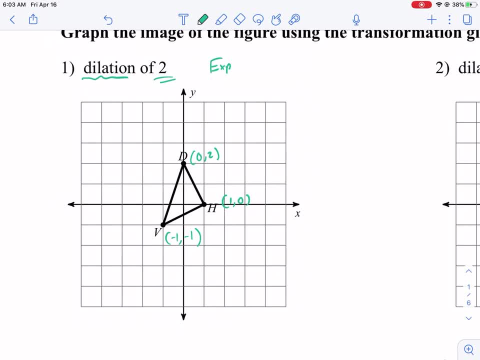 that mean. Dilation means it's either an expansion or contraction. So here it's going to be an expansion or it's going to be a contraction. So it's either going to get bigger or it's going to get smaller, And that's what it means. Now, dilation of 2, this is talking about. 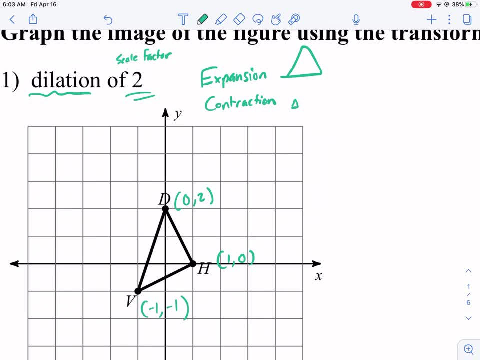 the scale factor. A scale factor is something that makes it either grow or shrink, So think expansion is grow. There's lots of words I've thrown out, but this is all synonymous And our contraction is shrink, And that's what the scale factor helps us determine. So if it's 2, if it's, 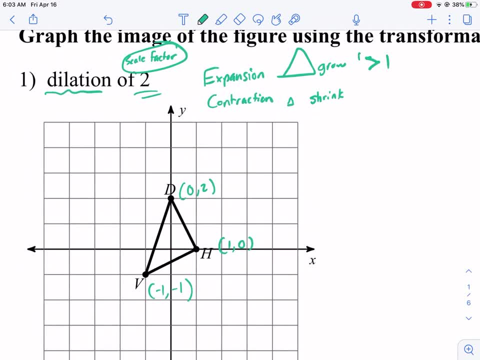 bigger than 1,. bigger than 1,, it's going to be an expansion, And if it's less than 1, it's going to be a contraction, It's going to shrink. If it's 1,, that means it doesn't change any size. So let's. 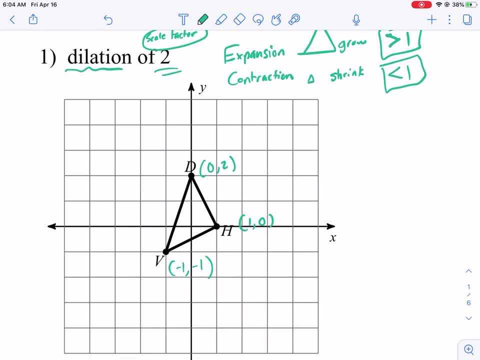 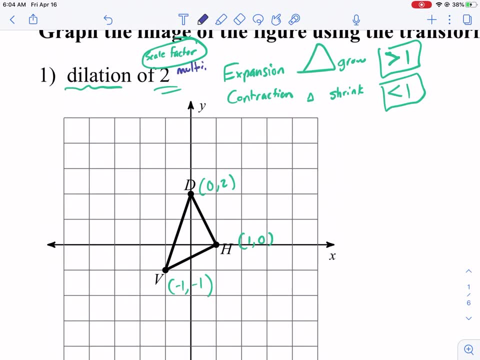 go ahead And take a look. If we're dilating it by 2, that means we are multiplying. So, scale factor: we always multiply by the scale factor, Okay. So what does that mean? We're going to take all our 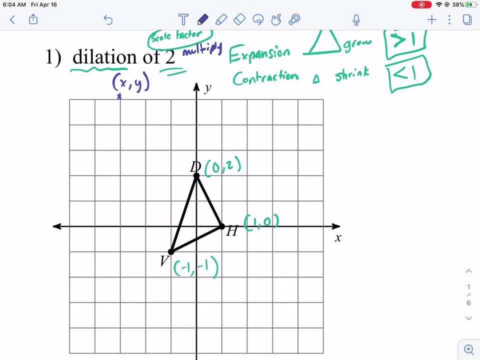 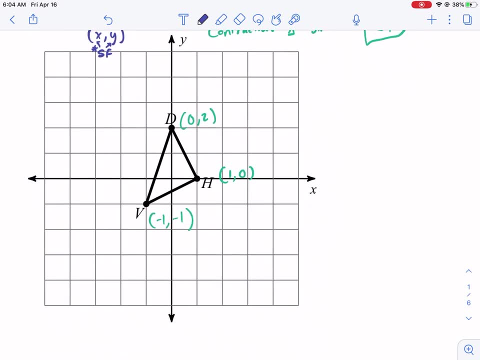 x's and y's and we multiply by our scale factor to the x and to the y, And that's what we're doing. So if we look at d, we're going to multiply both the 0 times 2.. 0 times 2.. 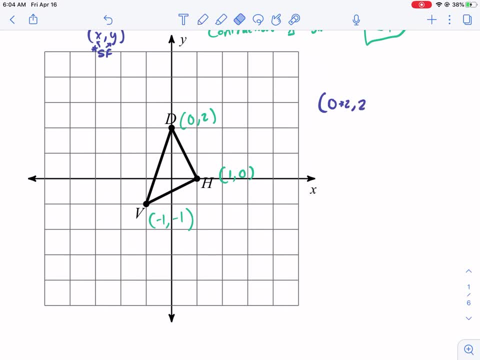 And the 2 times. I'm going to change it to a dot. I like the dot better- 0 times 2.. And then we're going to do 2 times 2 to get our d prime, And I'm going to write it off to the side first, before plotting it. For h prime, we're going to do 1 times 2 and then 0 times 2.. And then for v prime- all these primes are at the new location, by the way, So negative 1 times 2 and negative 1 times 2.. I'm going to highlight the scale factor. So there's scale factor dilation of 2.. 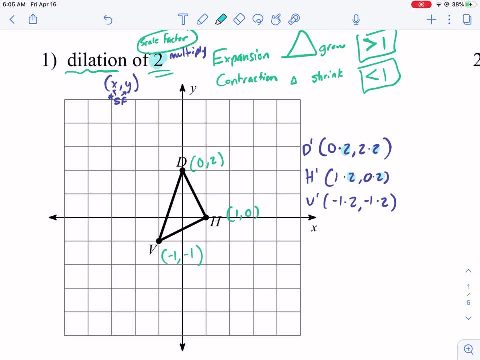 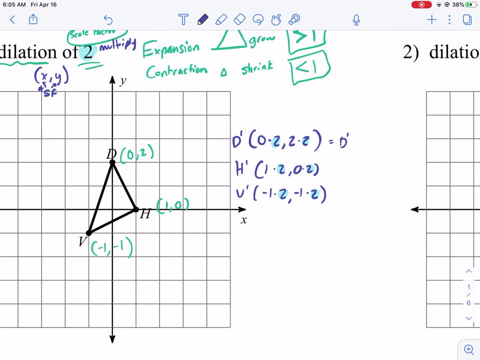 That's where that 2 comes from. We multiply the x and y coordinates of each by that scale factor. Now what is the new result of where this should be? Well, d prime is now going to be at 0, 4.. H prime is going to be at 2, 0. And then v prime is going to be at negative 2,. 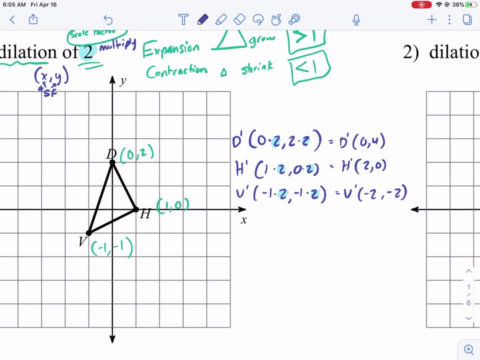 negative 2.. So we're going to go ahead and plot these new points. So 0, 4 is there, 2, 0 is there. negative 2, negative 2 is right there and we see that it has expanded. now it's a. it's a non-rigid. 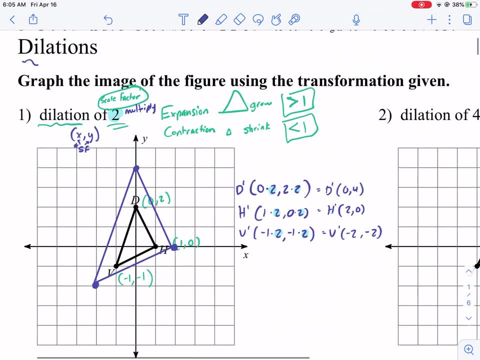 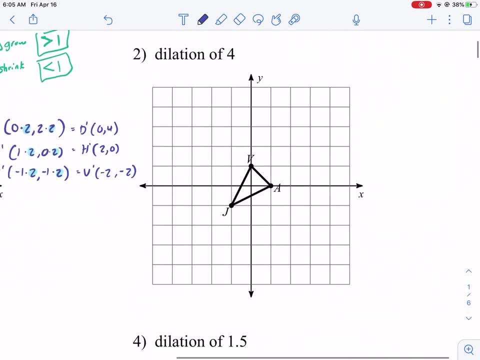 motion. that means it doesn't maintain its shape. that's what dilations are. they're non-rigid, meaning it doesn't keep the same dimensions. but it is the type of transformation. now, if we look at these ones again, we're just going to multiply by four. so i like to look at the coordinates first. 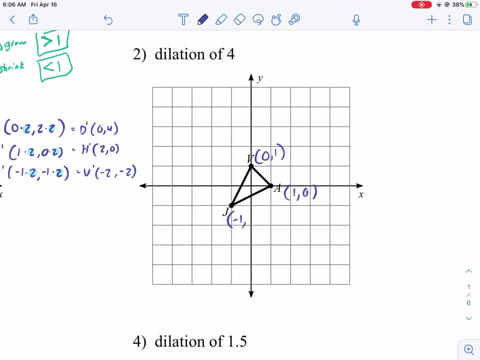 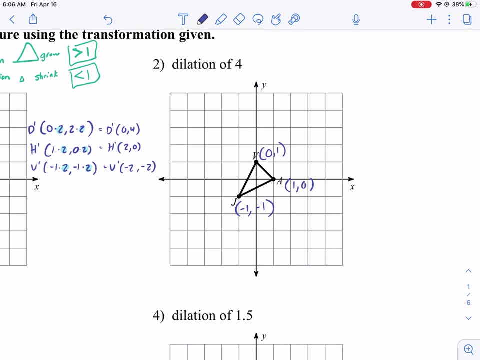 i think that's a super important part. we need to look at these coordinates and it looks like it's the same. oh no, it's not the same shape, exactly very similar. and we're just going to multiply by four. so zero times four is zero, and then one times four is four. so the new location. 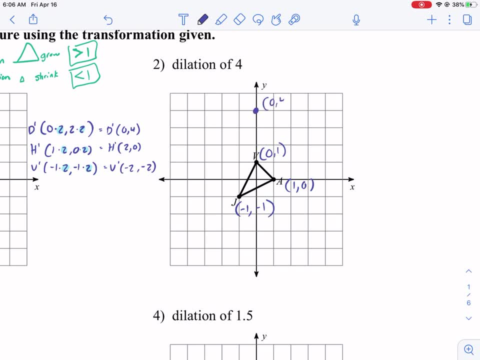 one, two, three, four is going to be here, zero comma four. then we go to one times four and that's four. one, two, three, four for the x value, and then zero times four is zero. so it's going to maintain, uh, that, right there, anytime it's zero. you know it's going to stay on that line, wherever it is. 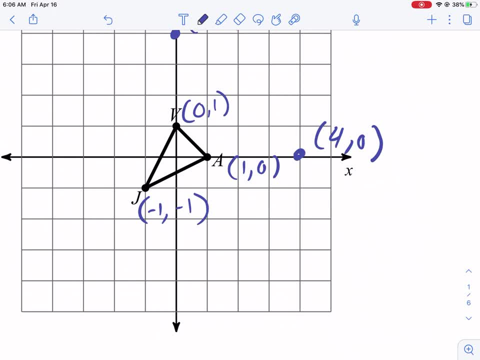 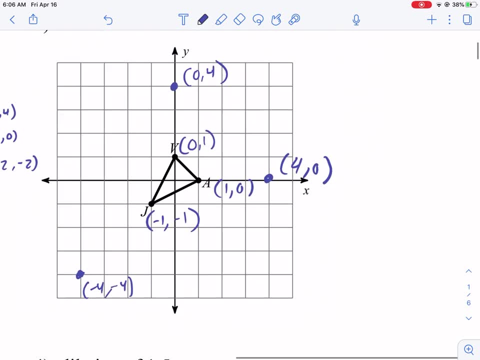 you, and then we have negative one times. four is going to be negative four. one, two, three, four. negative one, two, three, four. so it's going to be right here: negative four, comma, negative four after multiplying by four, and then we connect the dots and we're done. so it looks something like: 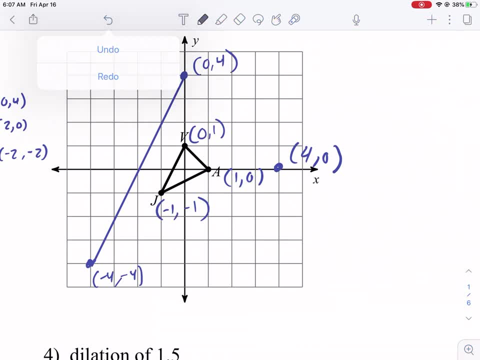 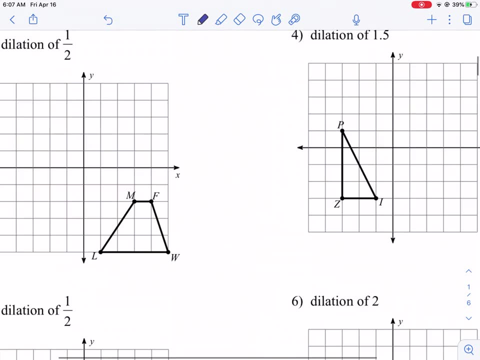 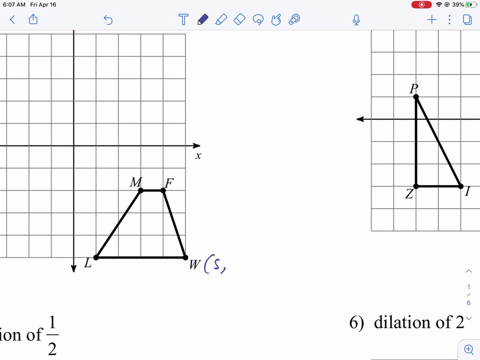 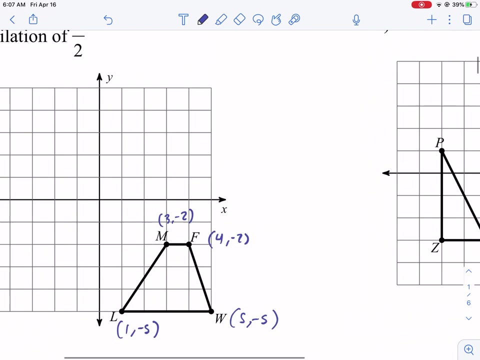 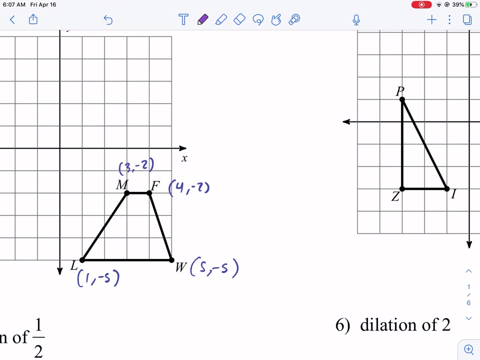 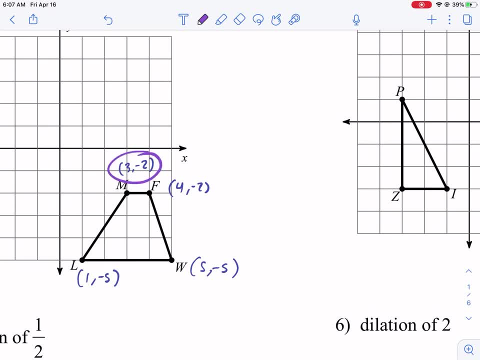 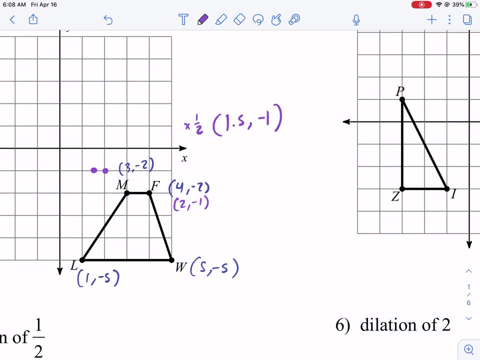 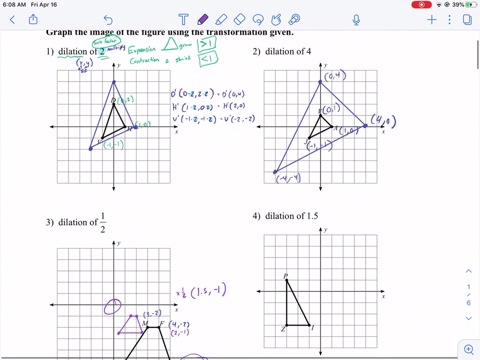 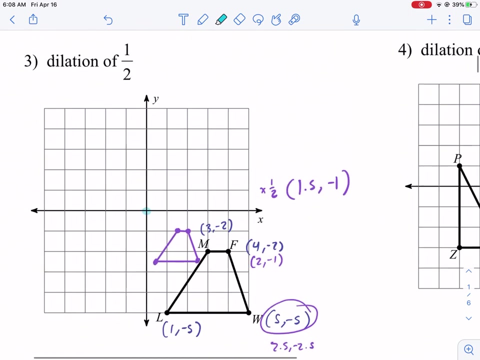 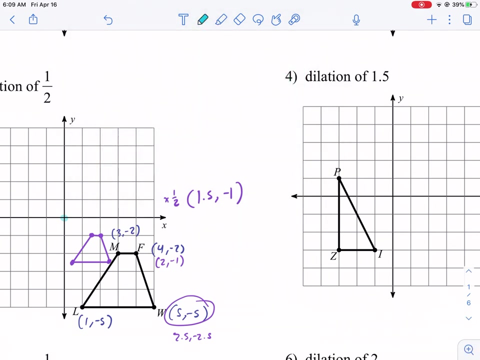 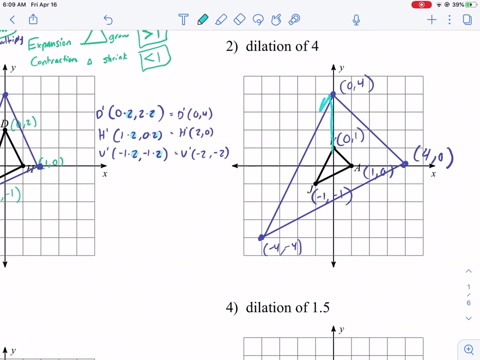 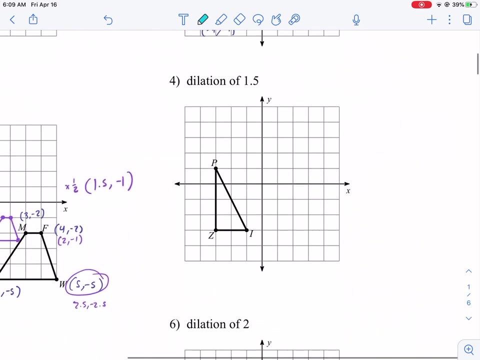 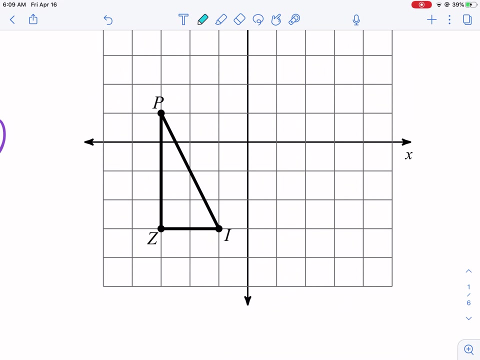 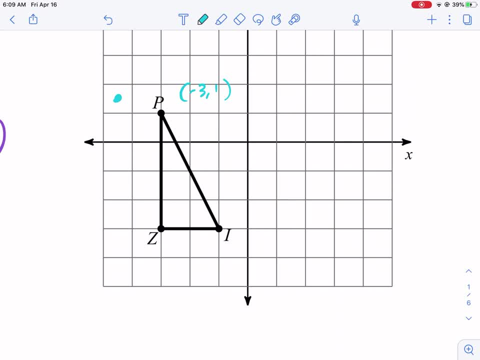 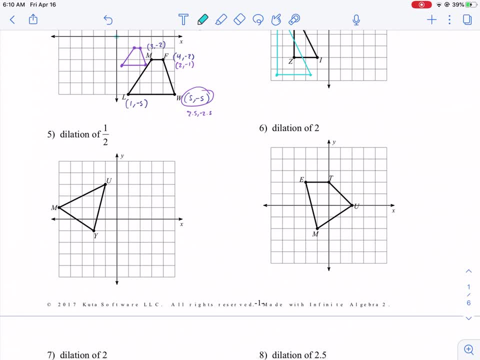 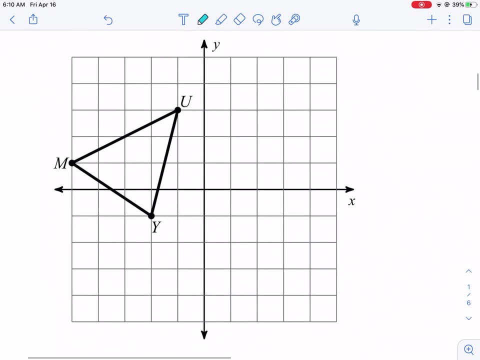 dilation of one half. same deal, it's going to shrink. i'll do this one because it's shrink, and then dilation of two. we just make it bigger, so it's going to be something like: it's up like that. so one half, i'll do this one. so this is here at. it's going to be 2.5 comma 0.5. 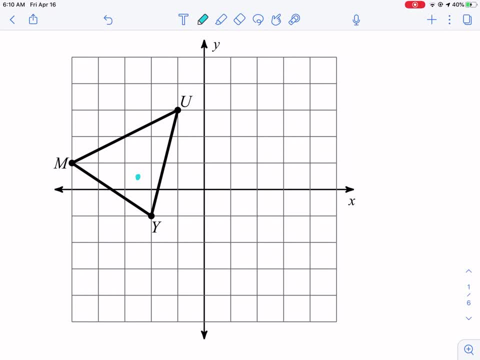 then we have negative one, uh, so it's going to be 0.5, and then three, so that's 1.5. and then we have this one which is going to shrink to 0.5, and then one. it's about here. so see how it has shrunk towards the origin. it gets closer and closer, closer to zero. zero as we dilate. 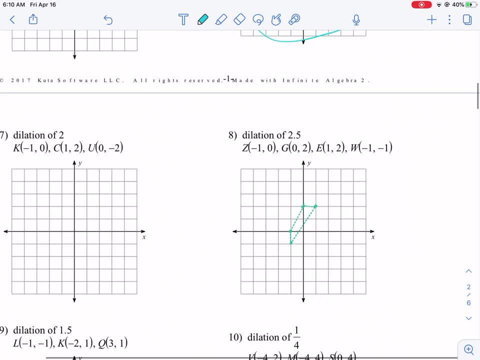 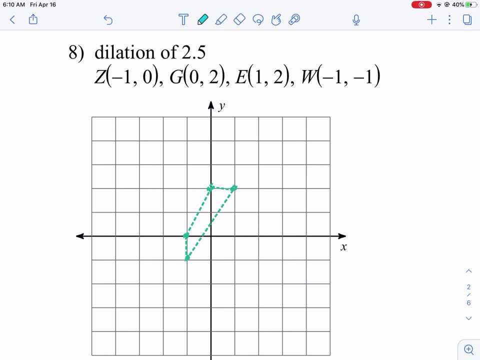 it, or shrink it now with these real quick. uh, these are coordinate. you can either plot them like i did with number eight and then expand from there. so multiply each one of these coordinates by 2.5. but since they already give us the coordinates, you might as well just go ahead and do that. 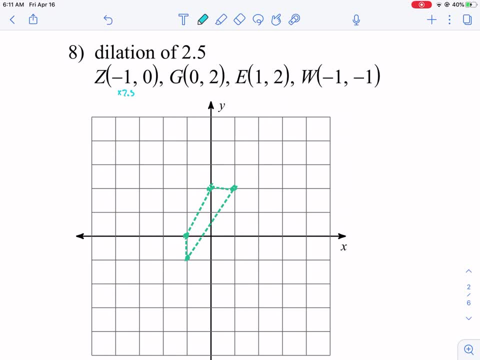 so I should have labeled z negative, one zero. so z is over here, multiplied by 2.5 and get a. 2.5 is what it's going to be, and when it stays at zero, zero two is going to expand to three zero three, one two. 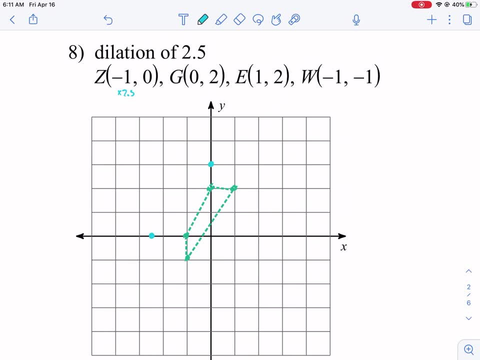 is going to expand to, uh, 2.5, so 2.5 and then two times 2.5. oh, i'm sorry, two times 2.5 isn't three. two times 2.5 is five, so i need to put that up to five. so pull 2.5 comma five, negative one, so we have negative 2.5. 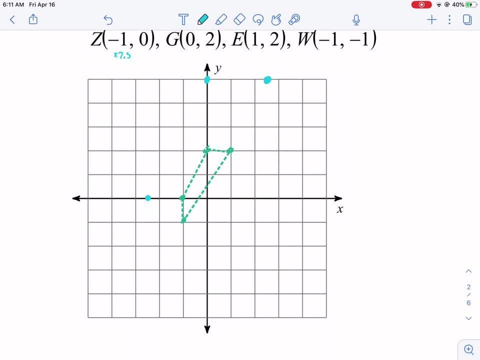 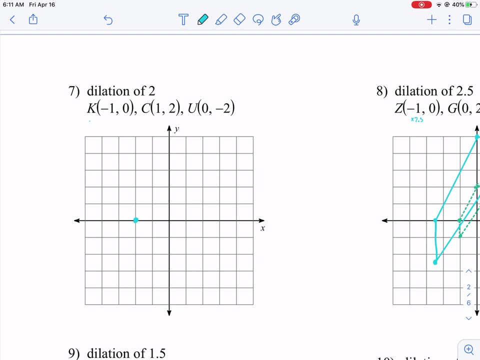 negative 2.5. and that is here, and we connect our dots. so this is a new image, okay. and then something as simple as, uh, this one: we just multiply each one of these by two, so we have negative two zero. i'm just multiplying all these coordinates by two and i have two comma four. 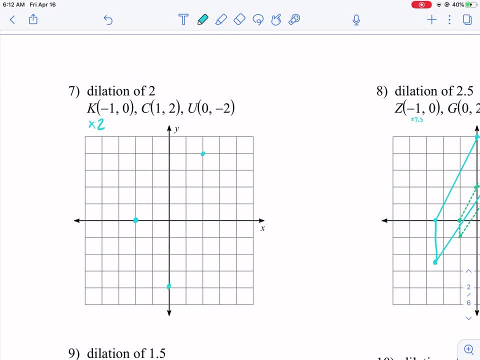 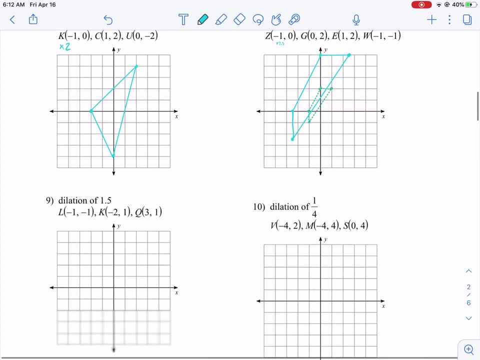 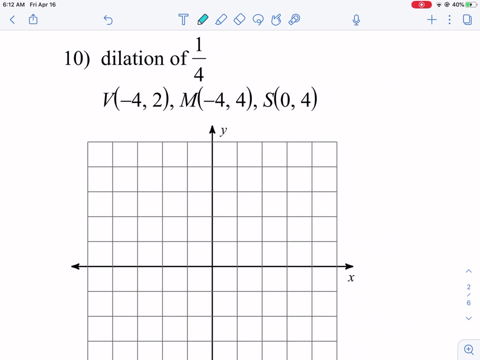 and i have zero comma negative four, and this would be my dilation. i didn't draw the original shape, but this would be my dilation because that's all it's asking for in this one and um, let's take a look at this same thing with hith. we're going to multiply by one fourth, so to get negative one. 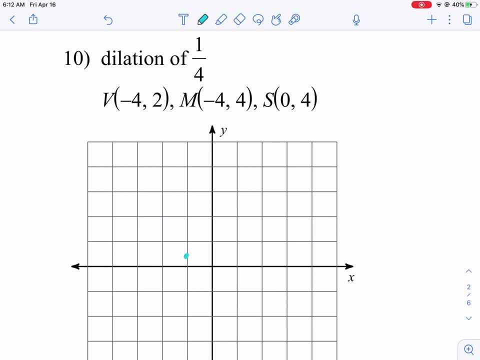 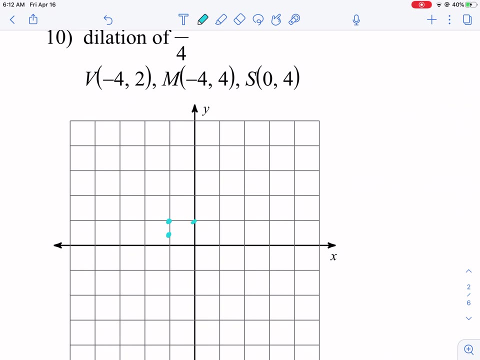 comma 0.5. right, so two times one over four, two over one, we get two. yeah, one half. okay, so i was right, just double checking. then we have negative one comma one, then we have zero comma one, so our shape gonna look like this after that: 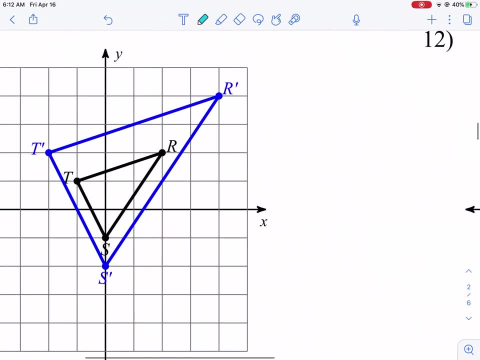 dilation is really tiny. now we have a rule, so what we have to do is we have to label each coordinate and then see how the x values change. so this is two comma two and it changes to four comma four. so how does it change between the x's and y's? well, it has to be the same thing. what? 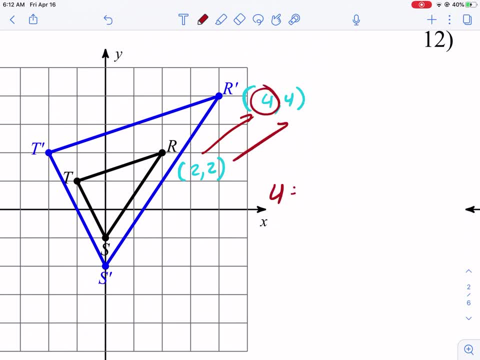 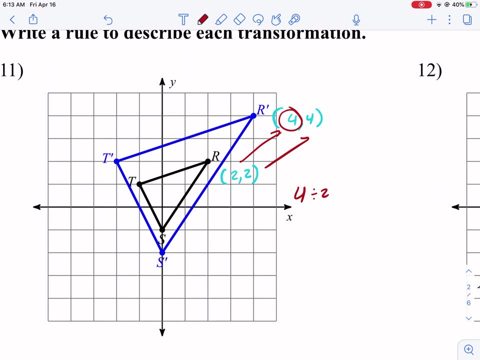 and what you can do is you can take the bigger one and divide. so you can do four divided by two, assume. oh, so no, we take the new image, the blue, okay, divided by the pre-image. So it might be a shrink. So then, 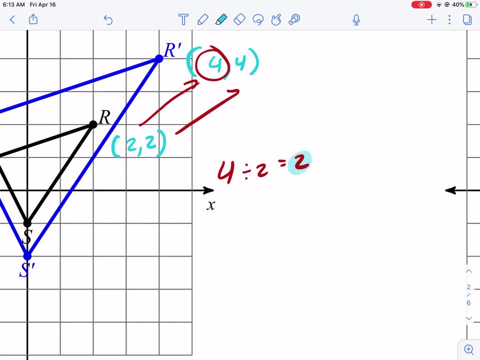 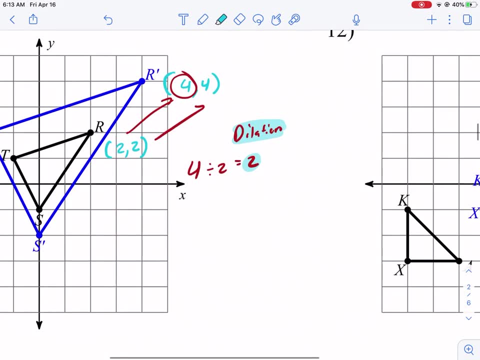 in this case it's a dilation. This is going to be our scale factor, So it's a dilation of two for this one. Okay, Cause we did four divided by two. two times two gives us four, And that's what it is. So, again, we take our new image. okay, Divided by the pre-image. 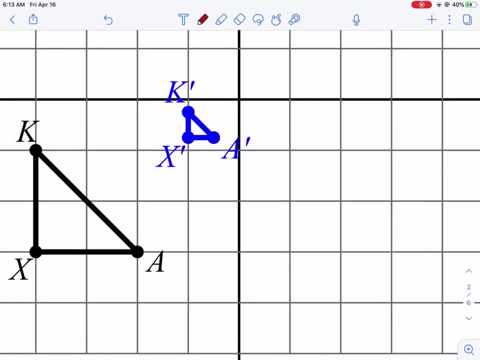 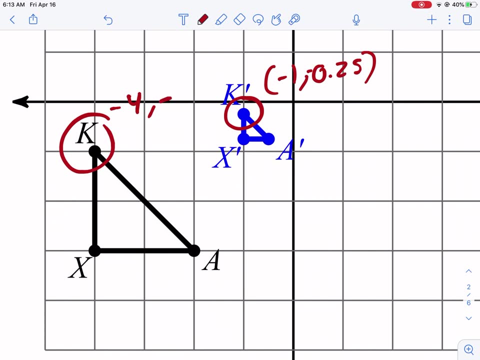 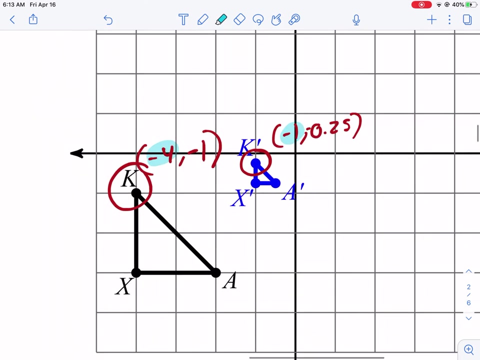 in this case our coordinate oof itty bitty, Um, it looks like that is negative one comma, negative 0.25.. And then this one is negative four comma, negative one. So really we just have to worry about the X coordinate. We don't have to worry about the Y coordinate that much, because 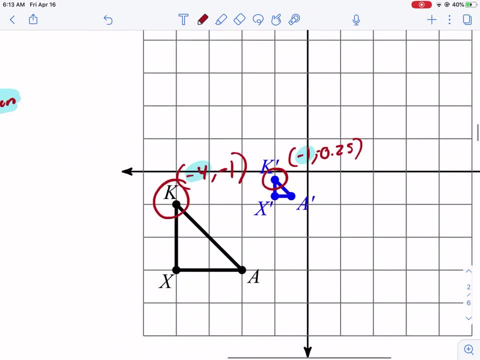 we want to look for whole numbers and it has to be the same for both X and Y, So we can do negative one divided by the pre-image, So we can do negative one divided by the pre-image, So we can negative four to find our scale factor. In this case it's one over four, So one fourth is our. 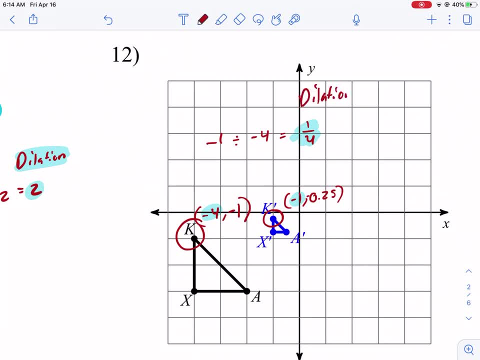 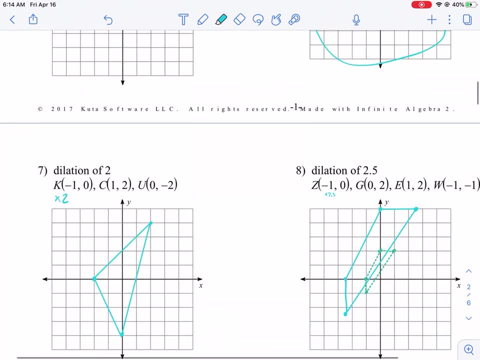 dilation for this one. So that's it. That's dilations. Hope you guys enjoyed this video. Make sure to check out Wes Explains Best for more videos on geometry or any other math concept. Leave a comment if you need something covered. Uh, and I hope to see you next time. right here on this channel. Thanks for watching.